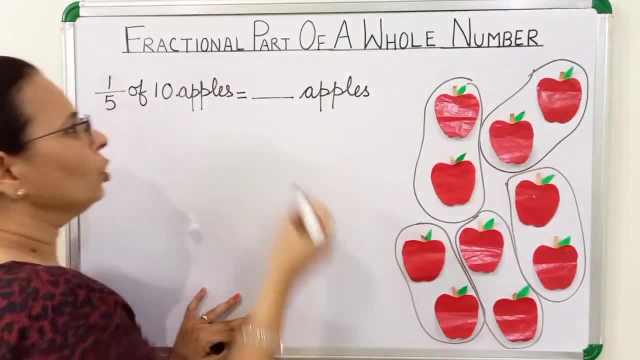 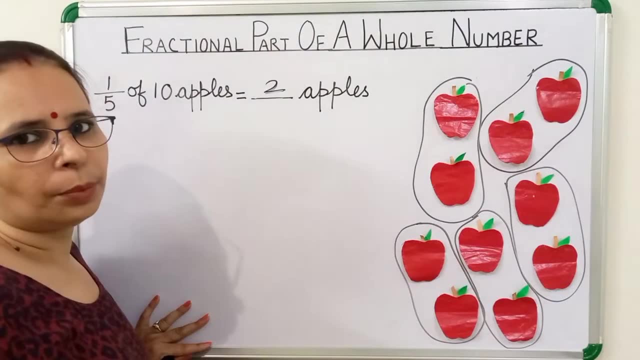 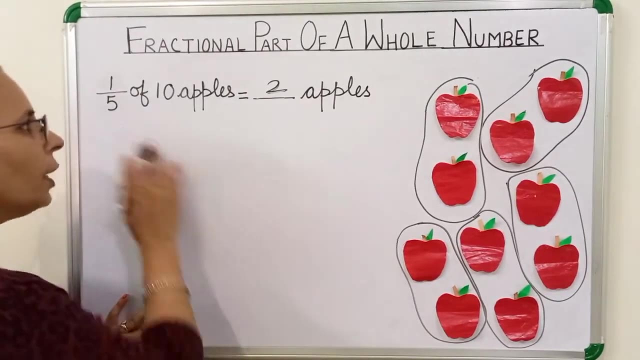 There are two apples in one group, So 2 is the answer. Now we will solve this sum in mathematical terms. In mathematics of representational math there is multiplication, So we can express this sum as 1 fifth multiplied by 10.. 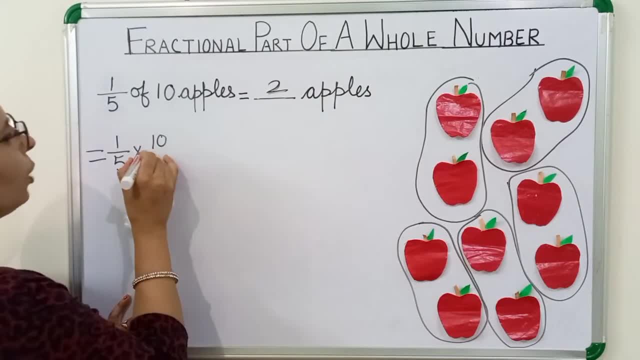 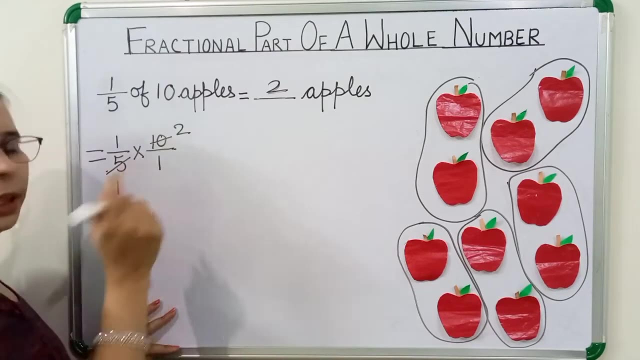 We will write 10 in fraction by putting 1 in denominator. 5 cancels 10 two times. Now we will multiply numerator to numerator and denominator to denominator. 1 times 2 is equal to 1.. 1 times 2 is equal to 2.. 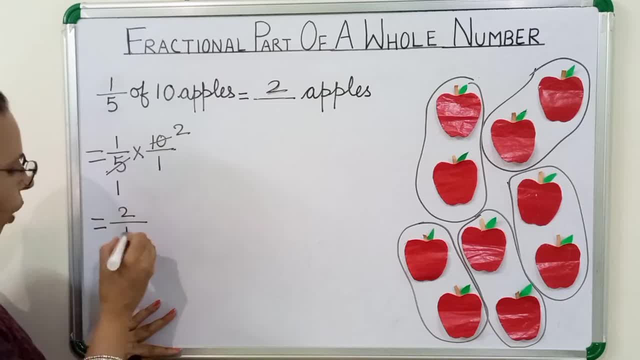 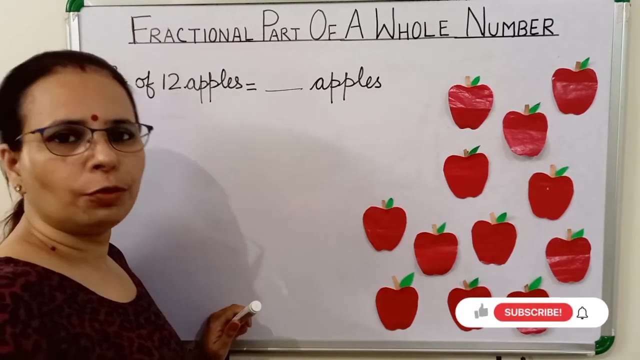 1 times 1 is equal to 1.. 2 times 1 is equal to 2.. Here we also get answer 2.. Now we will see one more example. We shall find 2 third part of 12 apples where denominator is 3.. 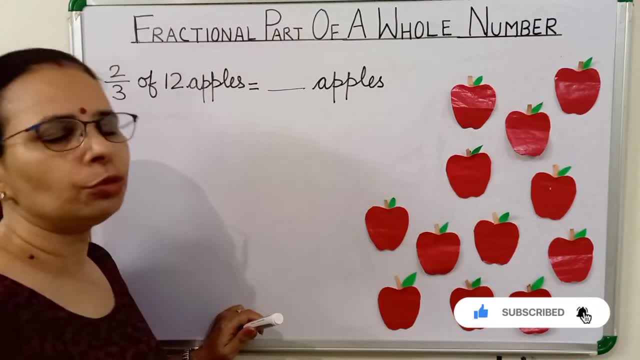 So we will divide these 12 apples into 3 equal groups. We will divide these 12 apples into 3 equal groups. We shall find 1 third part of 12 apples where denominator is 3.. As you know, 3 groups of 4 is equal to 12.. 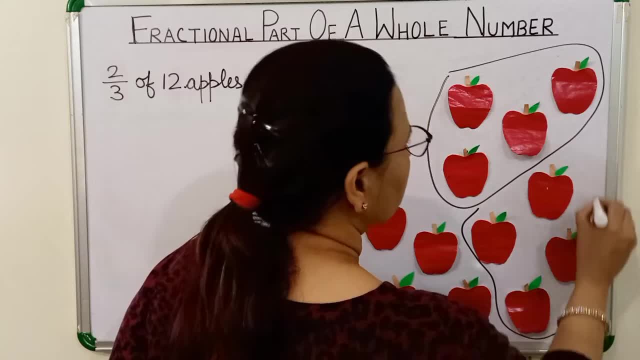 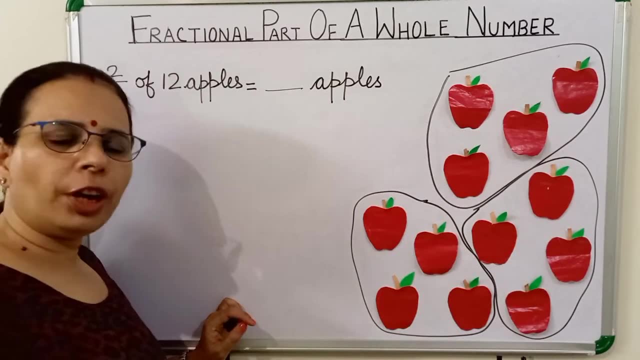 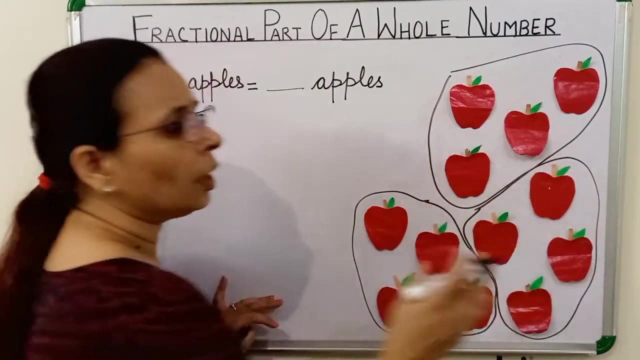 This is first group, This is second group And this is third group. We made 3 equal groups. Now we will see numerator. Numerator is 2.. So we will take 2 groups In 2 groups: 8 apples. 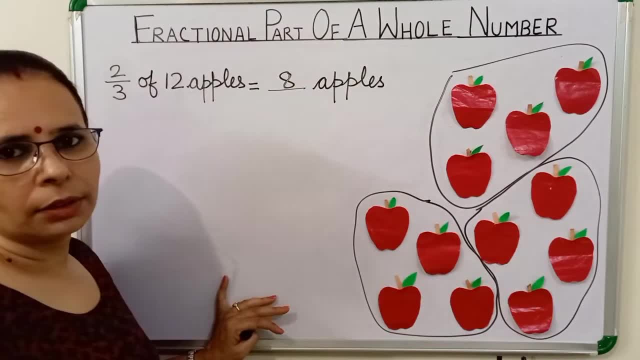 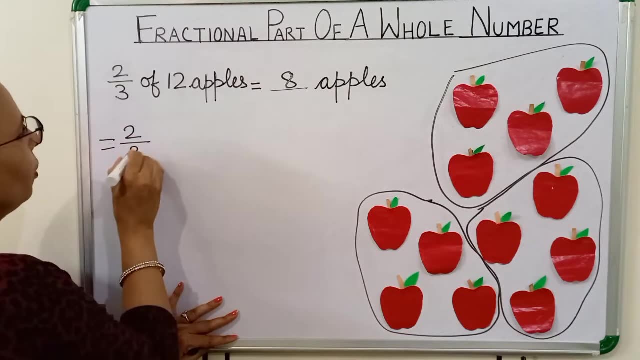 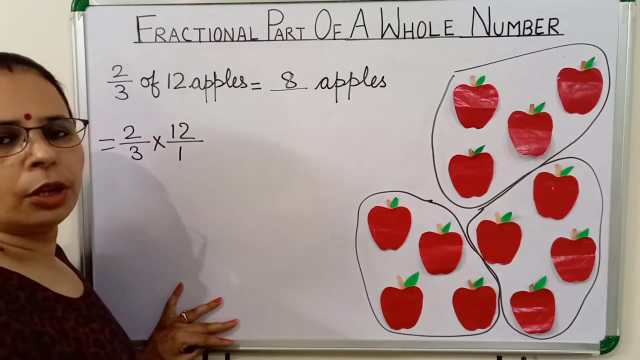 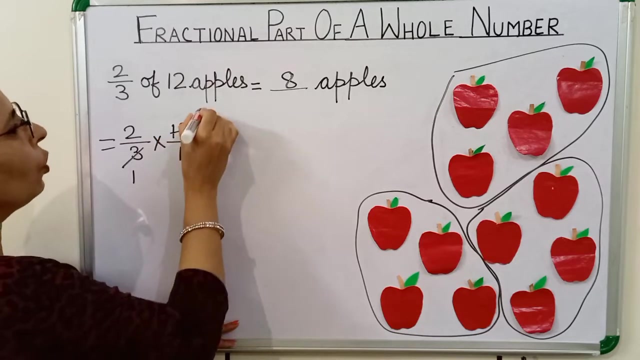 8 is the answer. Now we will solve this sum in mathematical terms: 2 upon 3 multiplied by 12.. We will write 1 in denominator to make 12 a fraction. 3 cancels 12 4 times. Now we will multiply numerator to numerator and denominator to numerator.